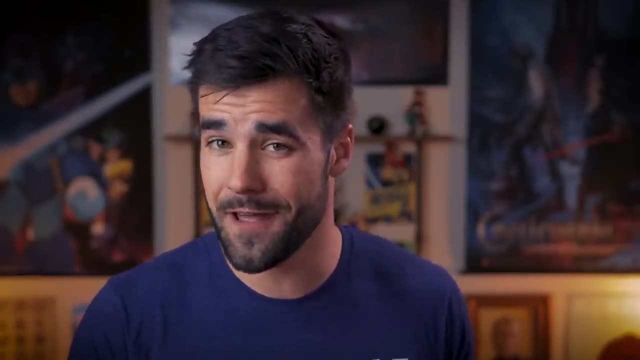 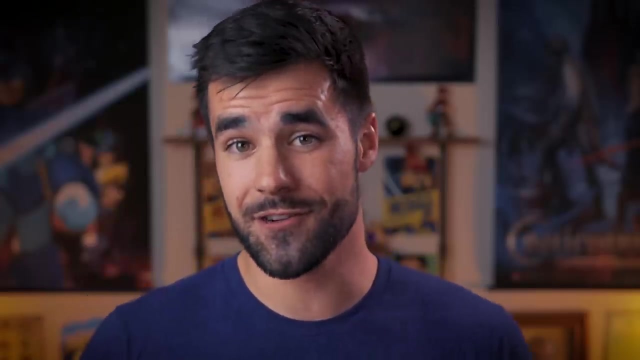 you can trust from one that you can't, from one that's probably going to fail you. Well, I think there's a few different criteria that we have to list out here. First and foremost, a system that you can trust is one that is not going to lose your data- This immediately. 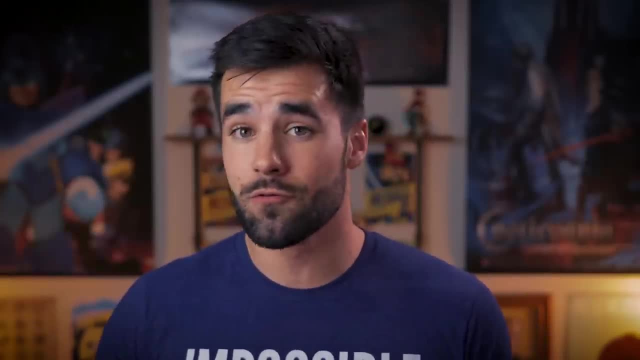 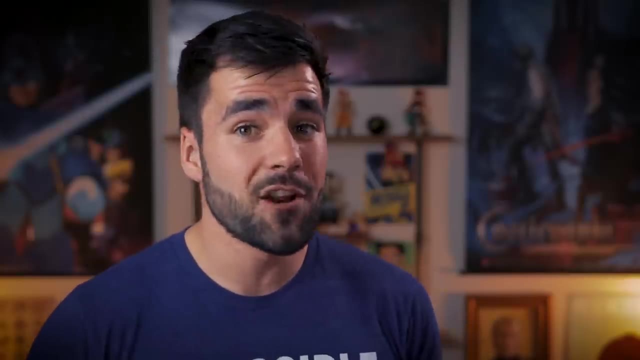 rules out your brain, because our brains forget things all the time. but it may also rule out a paper notebook if you don't keep that notebook backed up some other way, such as digitizing it. On the other hand, you've got systems that are designed with data retention. 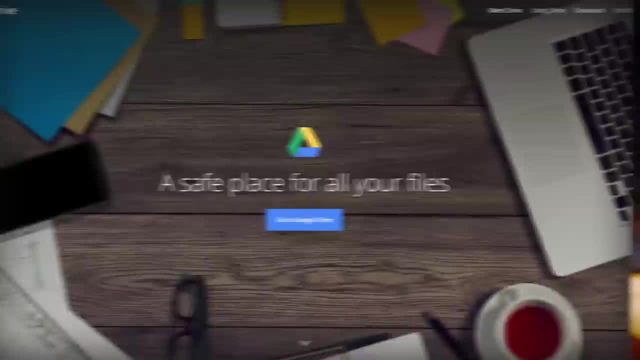 in mind Apps like Evernote or OneNote or Google Drive or anything else that has redundant servers across the world that make sure your data is backed up. So if you're looking for a system that you can trust, you can trust one that you can trust from one that you can't. 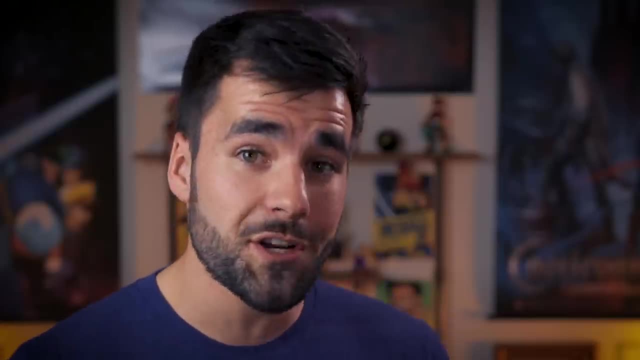 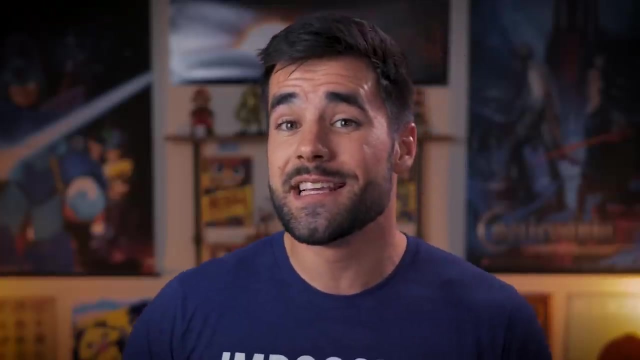 make sure your data is backed up and safe, even if the computer where you originally recorded that data ends up breaking somehow or gets burned up in a fire or is otherwise destroyed. Secondly, that system needs to be easily accessible. So if you do, really, 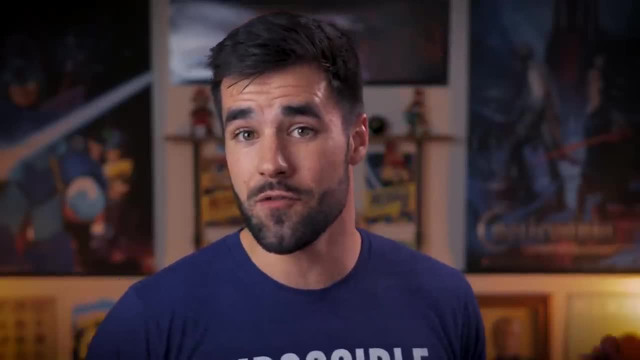 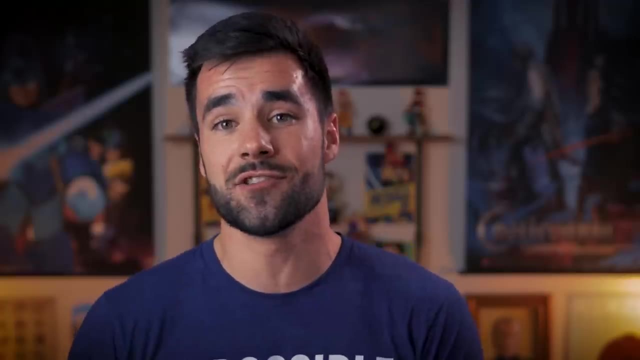 want to use paper, make sure it's a paper notebook that you are keeping with you wherever you go. Or if it's a note-taking system, make sure it's a cloud accessible note-taking system. so, whatever device you're using at the time, you can easily search it to find. 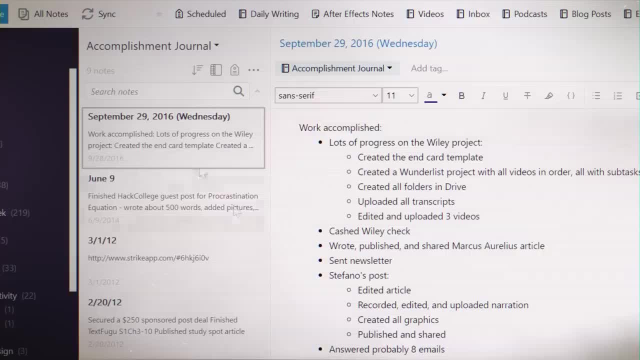 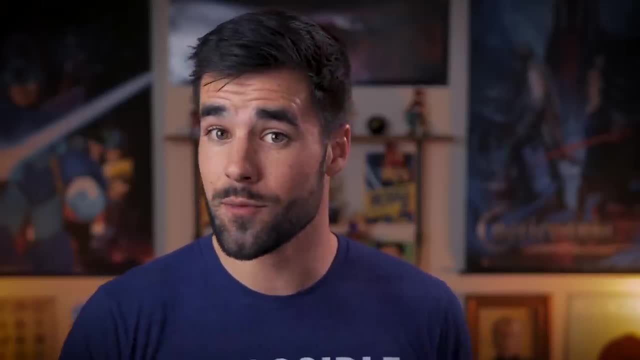 what you're looking for. Third, that system needs to be well organized itself and easily searchable. Make sure it has a map or tool you decide to use, make sure that it has a logical file or folder system, make sure it has a usable search tool and make sure your naming convention. 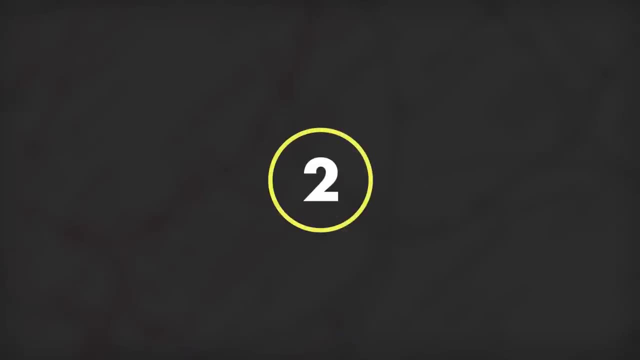 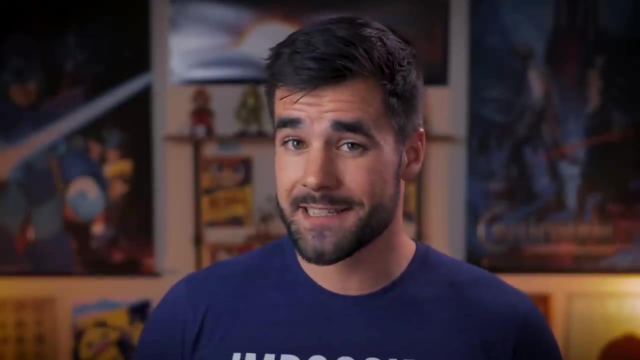 makes sense. Secondly, organized people make sure to label things, and they're especially diligent about doing this with things that they aren't going to use or interact with for quite a long time. To give you a very succinct example of this: the desk right next. 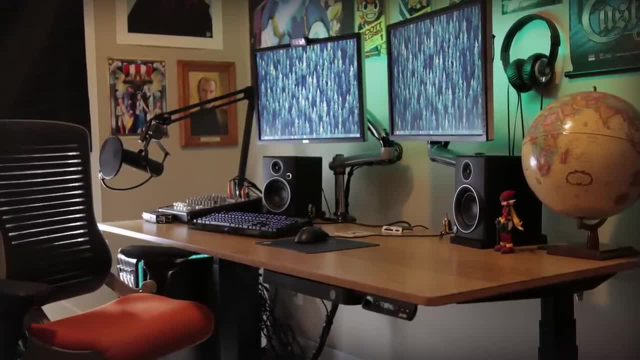 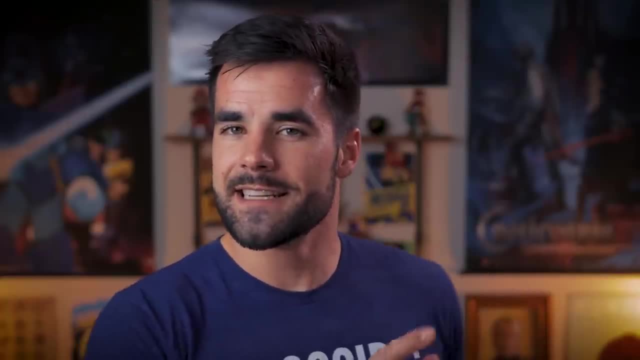 to me has some hardware that I almost never need to use, except for instances where I'm moving. So of course I've tossed that hardware in a plastic bag. it's in one of my cube organizers. it's safe and sound. But if I didn't label that plastic bag and I go maybe three years in between moves, I'm 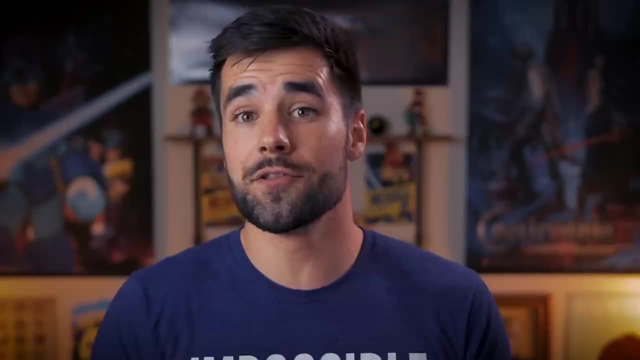 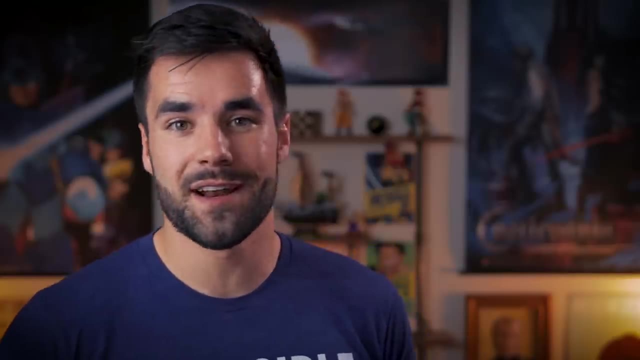 probably not going to remember exactly what that hardware is or what it goes to when I pull it out of that cube organizer and try to figure out what to do with it. And actually this is a pretty timely example, because I've got plans to move out of this apartment in. 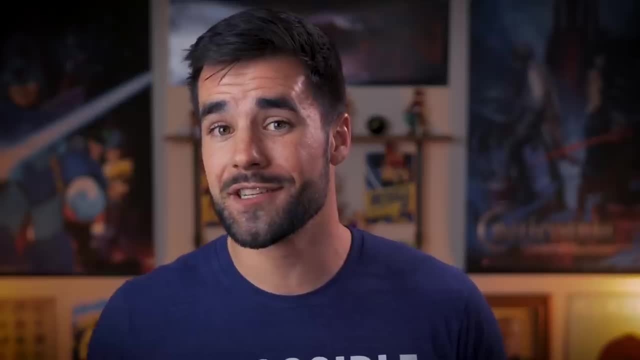 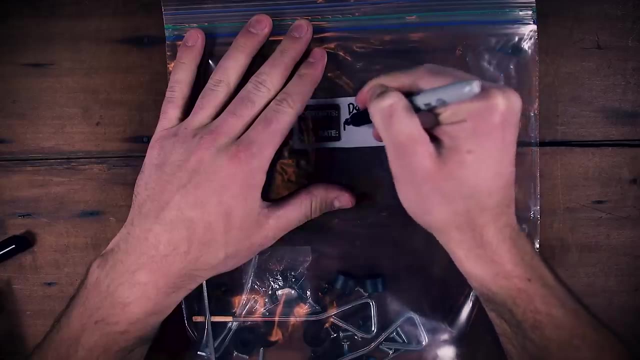 just a few months. But luckily my past self thought about this and remembered to buy plastic bags with little label areas. So last time I was moving and I put all that hardware into that plastic bag, I remembered to write down that this hardware goes to my desk. So when 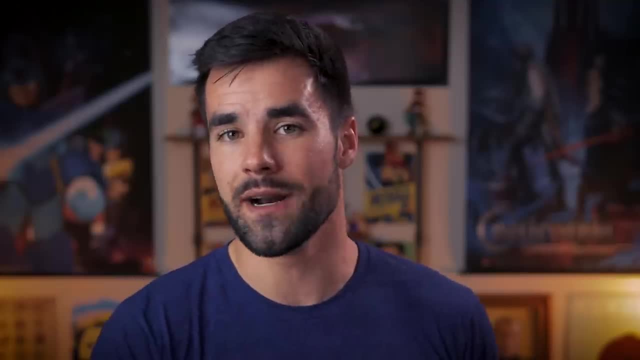 I go to move in a few months. I'm going to have to move it to my desk, So I'm going to use it in a few months. it's going to be very easy to find it and I'll know exactly what it's used for. 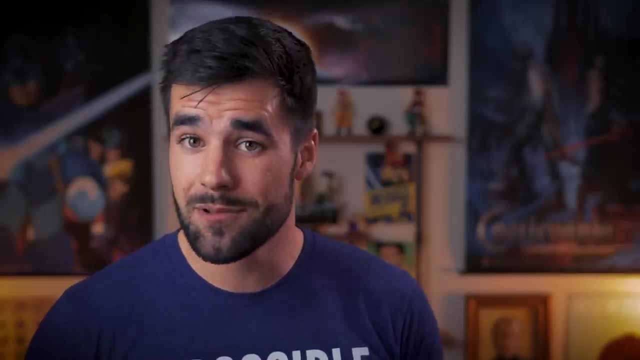 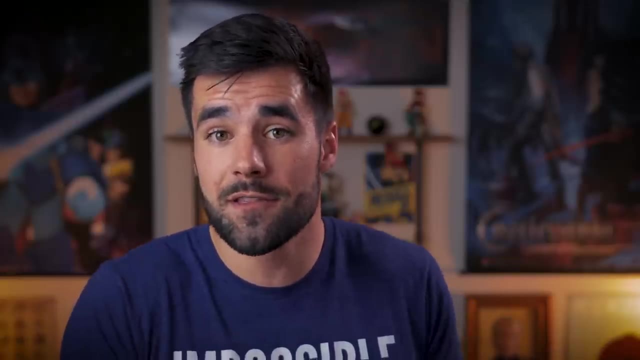 Now, this is just one example, and there are probably other things in your life that you should be labeling besides just plastic bags. For example, if you have one of those physical hanging folder organizers, you probably want to use the labels that it comes with to write. 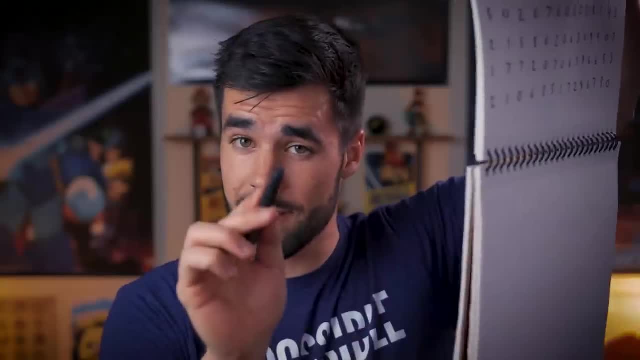 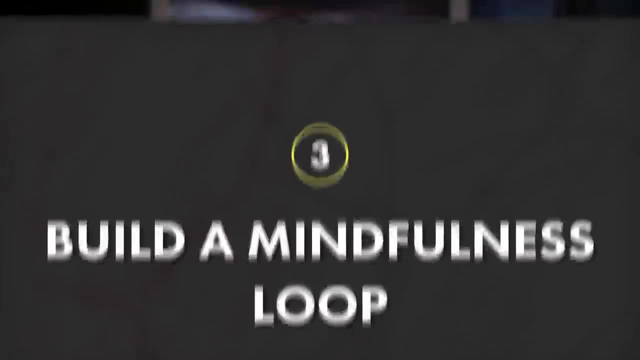 down what should be going in each one of those folders. Item number three: organized people build what I like to call a mindfulness loop which constantly goes through the different dependencies in their lives and basically checks up on them. What exactly is a dependency? Well, it's pretty much what it sounds like. I'm going to give you a really simple example here. So every single organism in existence, down to the most simple single cell prokaryotic blob, has things that they depend on. For example, our little blob creature needs a watery environment. 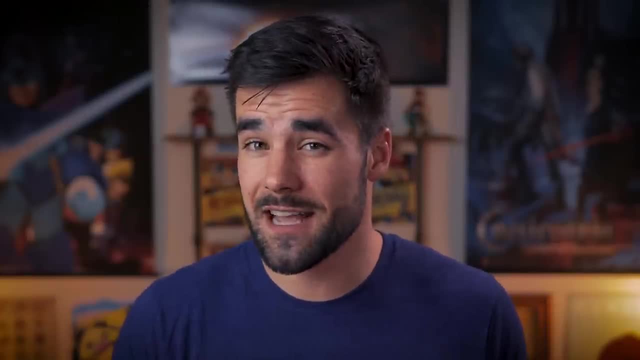 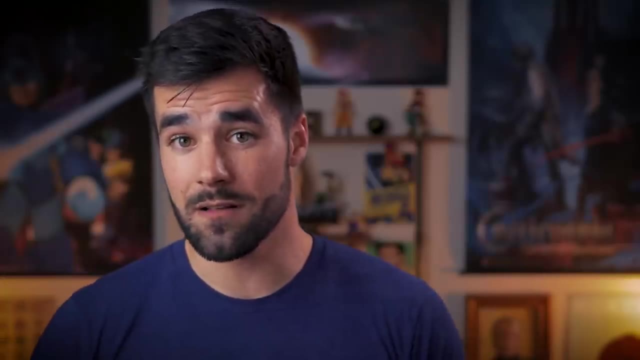 to move around in and a food source. It doesn't have a whole lot of dependencies in its life, but there are still dependencies and without them it will die. And what is true for our blob is true for you as well. except for that you're a much more complicated organism and you have a much more complicated life With me. I'm going to give you an example. Item number four: organized people build what they like to call a mindfulness loop which constantly goes through the different dependencies in their lives and basically checks up on them. So every single organism in existence, down to the most simple single cell prokaryotic blob, has things that they depend on. For example, our little blob creature needs a watery environment to move around in and a food source. It doesn't have a whole lot of dependencies. 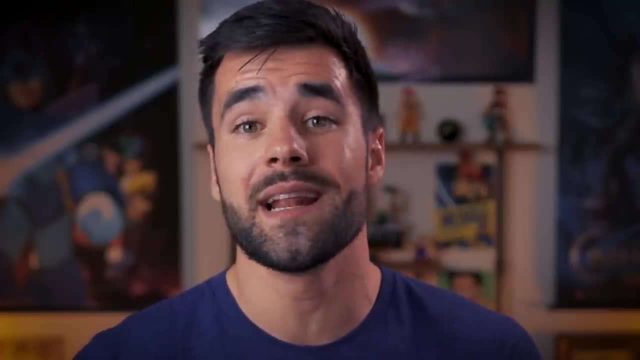 in its life, but there are still dependencies in its life, and that's where organized people build what they like to call a mindfulness loop. You have a lot more dependencies. You have your food, your shelter, your academic goals, your relationships. There are so many. 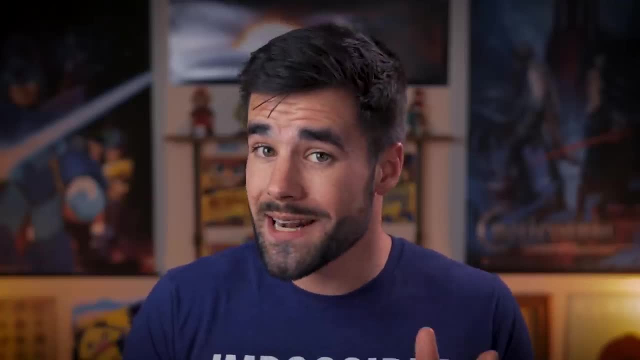 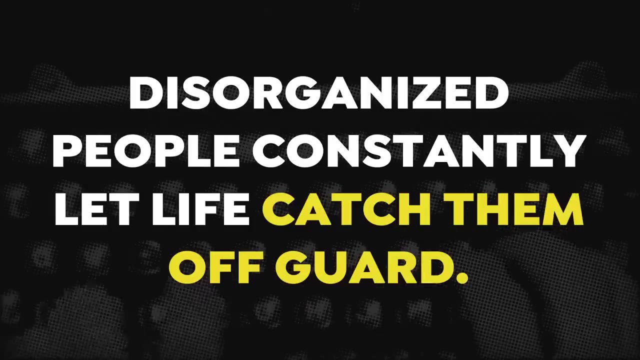 things to keep track of. And here is where one of the biggest differences between organized people and disorganized people can be found, because disorganized people are constantly being caught off guard by one of their dependencies and needing maintenance, needing action from them And, on the other hand, organized people are constantly looking ahead and figuring. 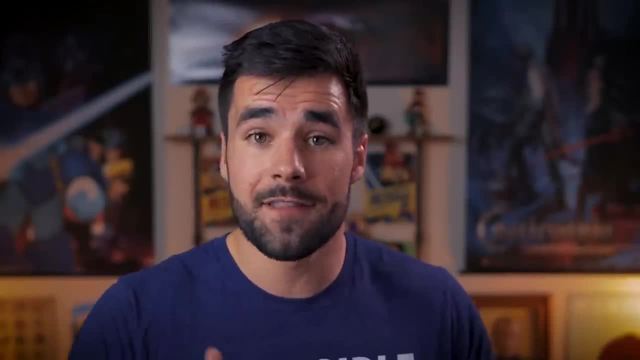 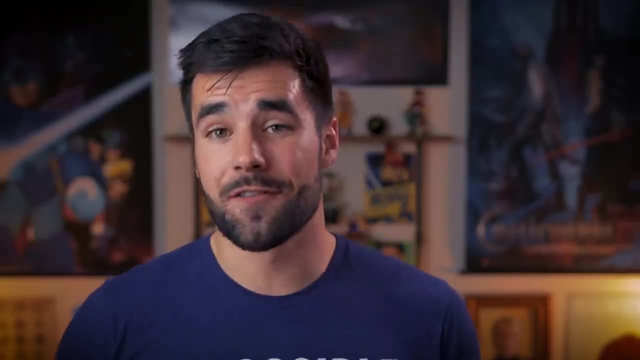 out what those dependencies are going to need in the future. They have this mindfulness loop constantly going on in the back of their mind. My absolute favorite example of a mindfulness loop in action actually comes from my mom. This was a story back from when I was probably 14 or 15 years old, I think I was up in my 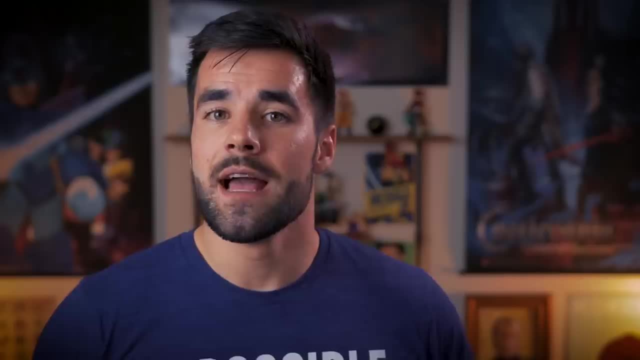 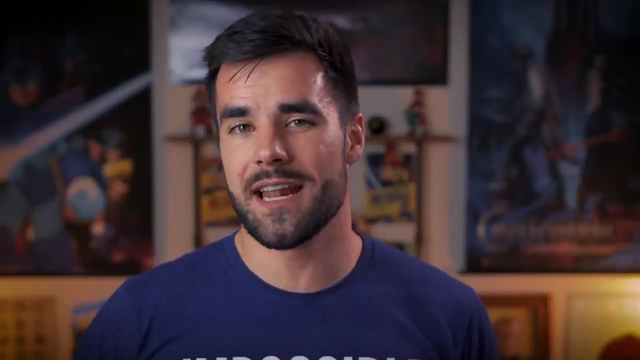 room on the computer just doing something that a 15-year-old does on a computer, and I heard her shout out to me: have you brushed your teeth today? And this was like at 2 pm in the afternoon. She was doing something completely unrelated to teeth brushing and 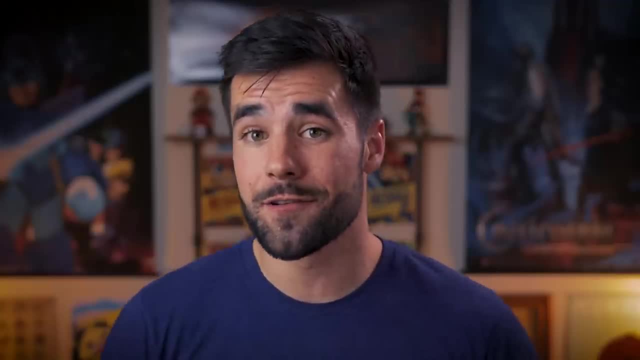 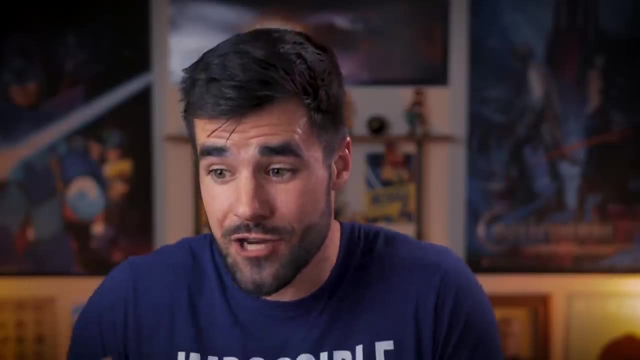 yet she thought to ask me Why, Well the heck? Because the health and well-being of her children were one of her main dependencies, and because my mom is an organized person, she got this regular mental notification to check up on that dependency. Now, admittedly, this is one of those mental patterns that 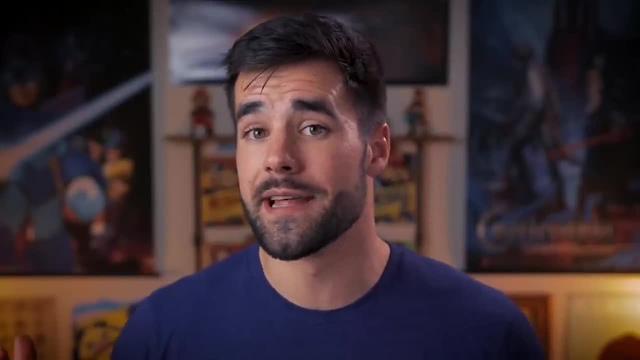 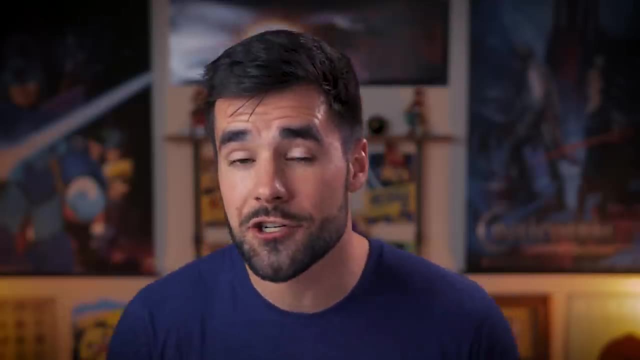 does take a lot of time and effort to build. You're not going to be able to flip it on like a switch, But I think the first step to building this mental pattern, which is incredibly useful, is to sit down and consciously list out your dependencies, Maybe even sit. 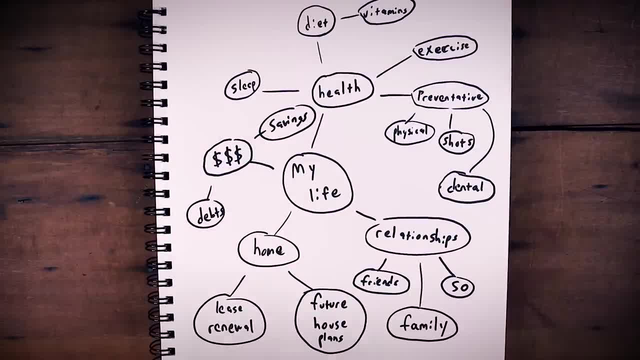 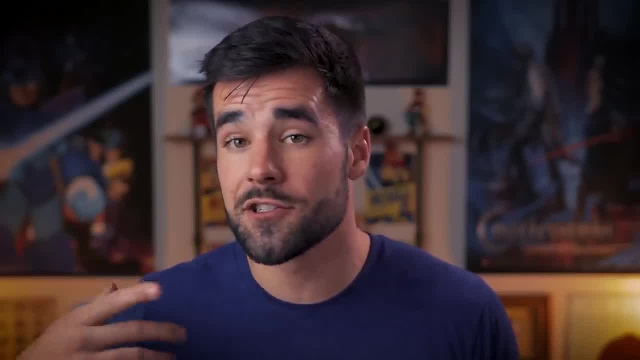 down and draw a mind map of all of your life's different dependencies And with this application of conscious thought to all the different aspects of your life, over time it's going to sink into your unconscious and you're going to start building that loop. 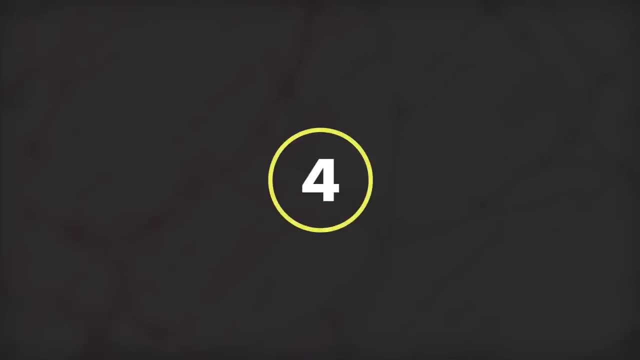 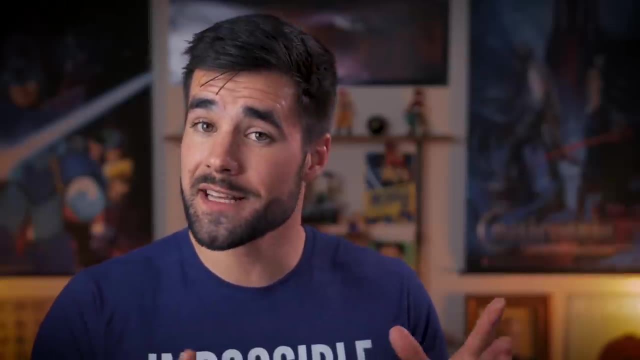 Item number four. Organized people live by the mantra: two is one, one is none. Essentially, this translates to have a backup of anything that you use on a regular basis, especially if running out of that thing in the middle of your work would hamper the rest of your. 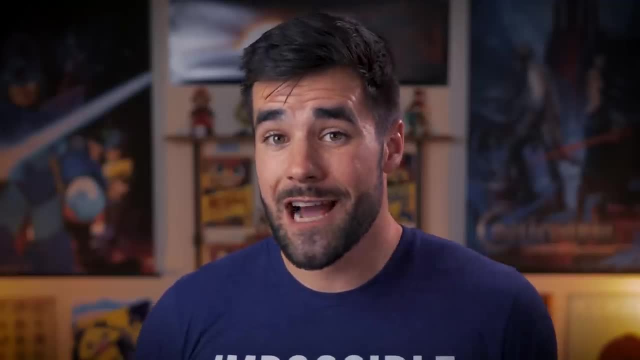 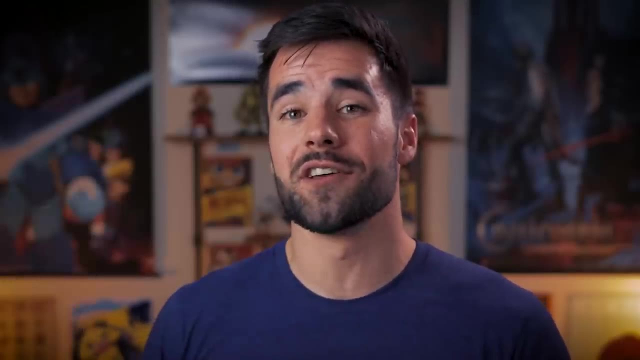 day or screw it up. For example, the camera that I'm filming this video on right now relies on a battery to run, And if that battery were to die during filming? well, luckily for me, I have an extra battery that's always on the charger on the wall, always fully charged. 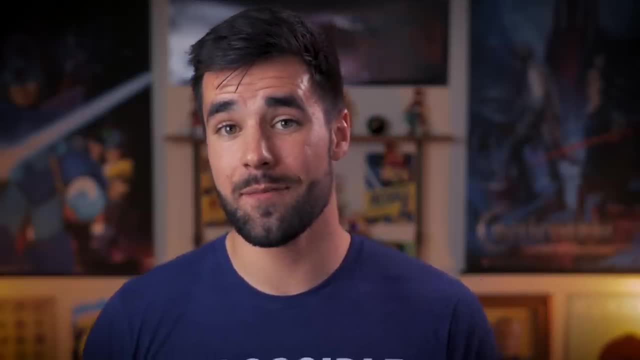 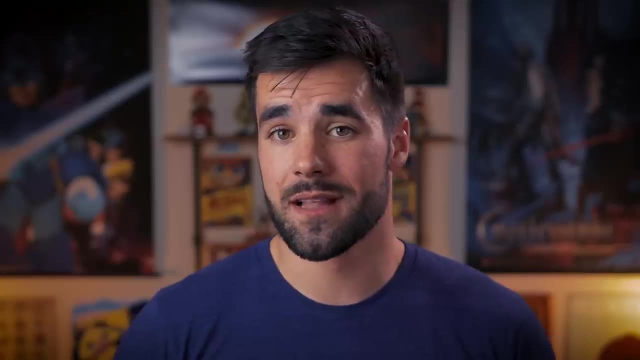 ready to go, because two is one and one is none. If the battery ran out and I didn't have the backup, I wouldn't be able to film and I might not even get a video out on time. And the same goes for many other things in my life. Memory cards I've got many, many 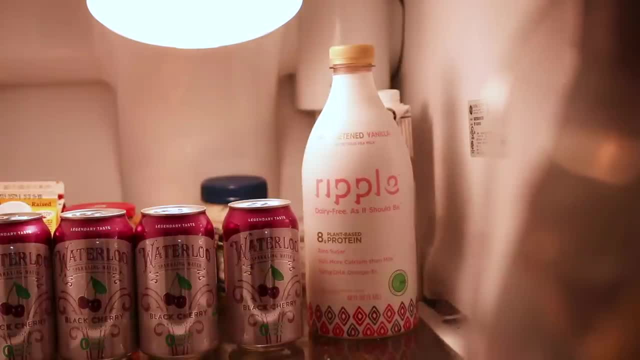 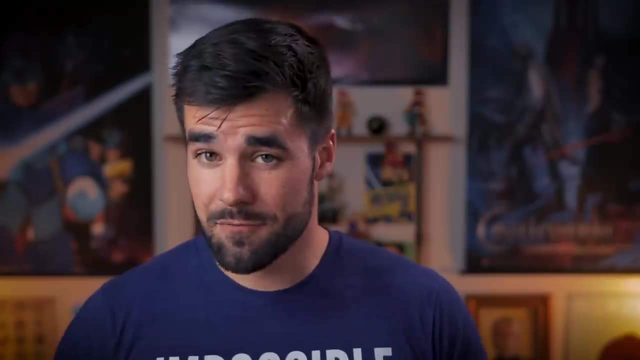 backups, Smoothie ingredients. well, there are two jugs of milk in my fridge instead of just one. That way, if I run out of one while making a smoothie, I've still got milk to use and I don't have to abstain from my smoothie that day. So just remember if running 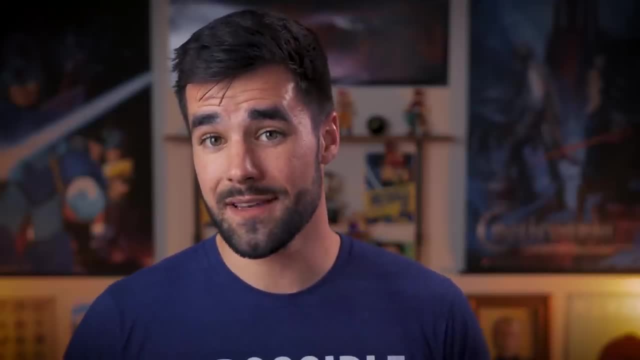 out of something while making a smoothie, I've still got milk to use and I don't have to abstain from my smoothie that day. So just remember: if running out of something would cause an interruption in your life, make sure you have a backup of it That way. 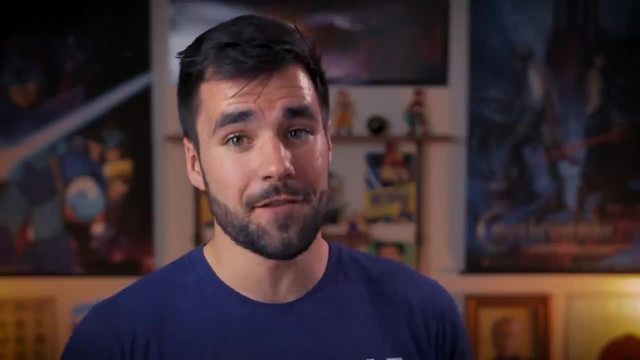 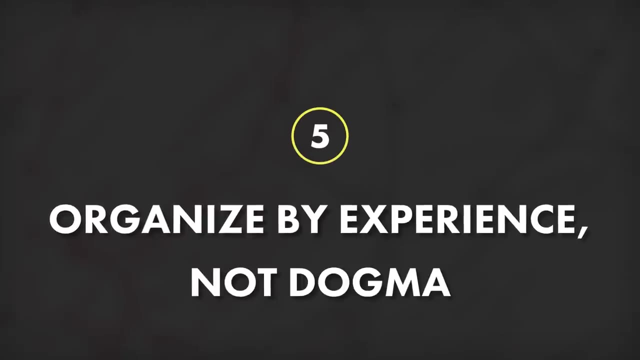 you can use the backup, go on with your day and then replace it when it is convenient for you to do so. Item number five: Organized people set things up in a way that is useful to them and that works, based on their own experience and experimentation. 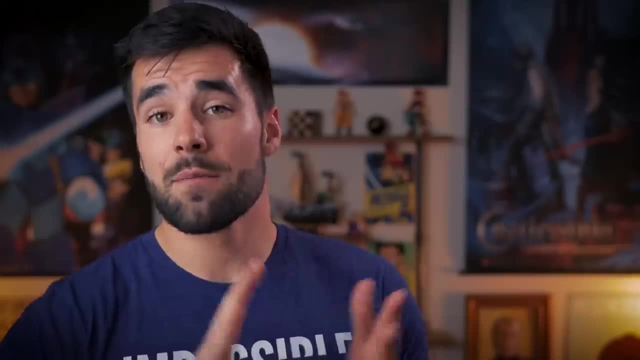 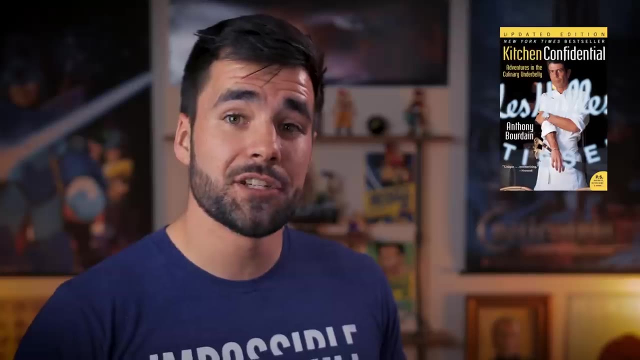 not simply based on dogma or how other people do things. Now, my favorite example of this principle comes from one of my favorite books, which is Anthony Bourdain's book Kitchen Confidential. In that book he talks about how many chefs inventory all the stuff in. 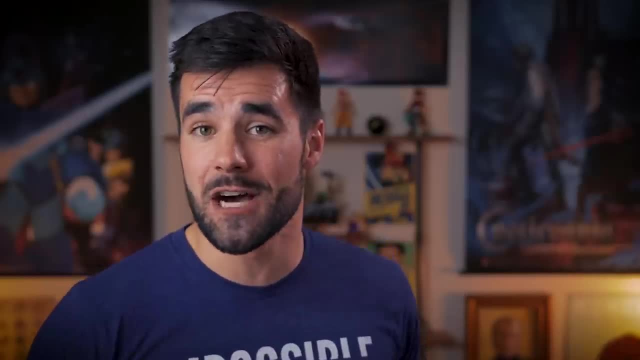 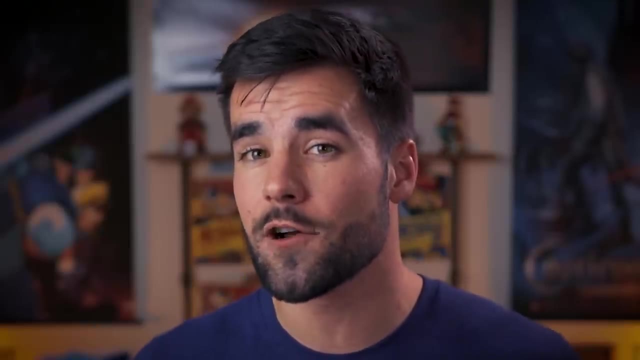 their kitchen alphabetically because, well, it just seems like the obvious way to create a list. But he didn't. Instead, he organized his inventory sheets so that the order of the items mirrored the geographical location of everything in the kitchen. And this actually. 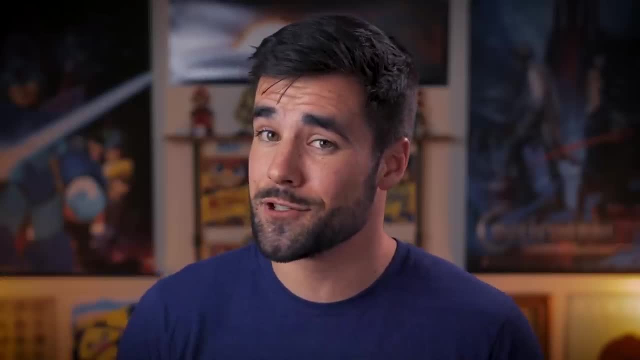 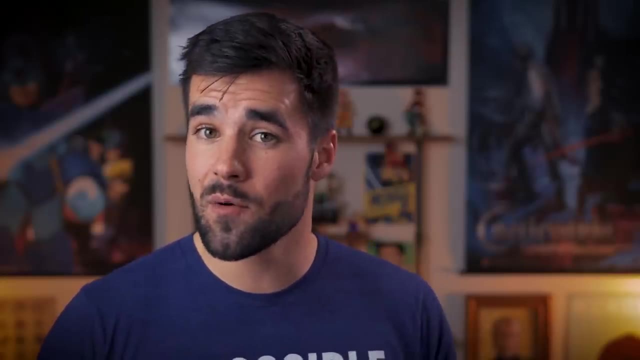 makes a lot of sense when you think about it, But of course, not everything that people do is based on sense. So ditch the dogma if it doesn't make sense. Question the established ways and constantly experiment with your processes and the way that you organize things. 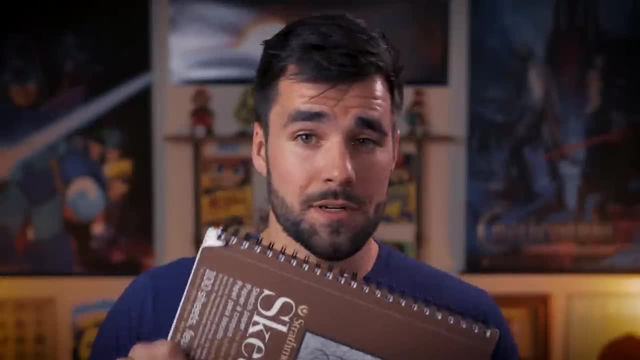 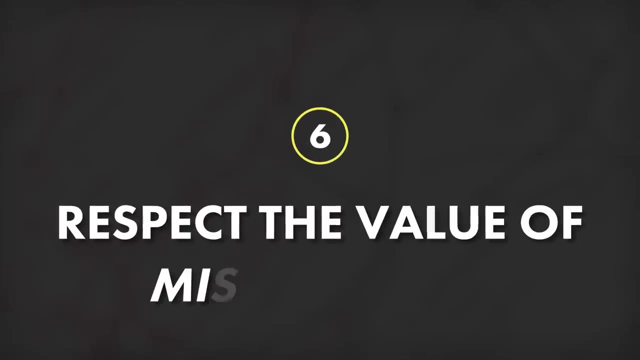 so you're doing things as effectively as you possibly can. Item number six: and I have run out of stupid things to do with this notebook prop. Organized people respect the value of mise en place, And this is a French term that roughly translates. 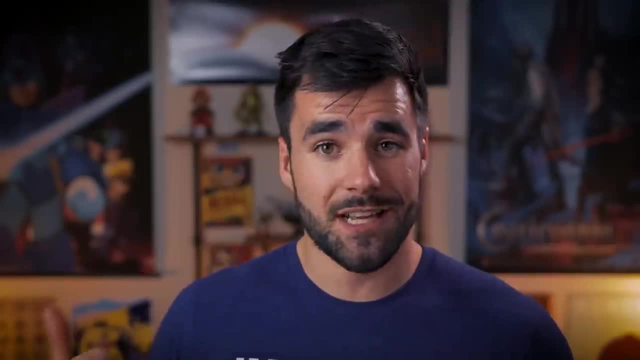 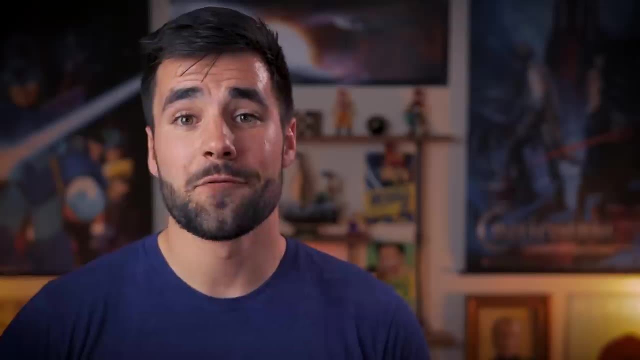 to everything in its place. To call back once again to Kitchen, Confidential Bourdain describes mise en place as your setup, your working environment and, to some degree, your state of mind as well, And within the culinary world, this is one of those concepts that every single 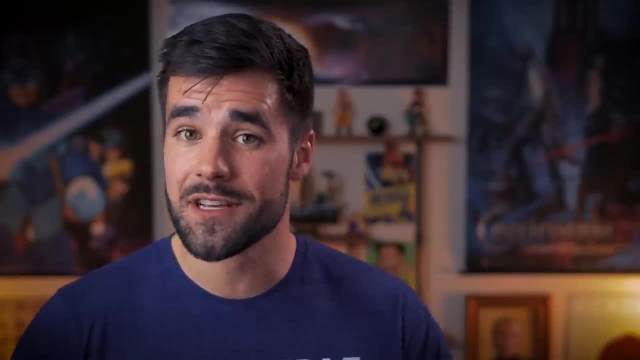 competent chef and line cook swears by, because to not use it, to not respect mise en place would mean to work in the kitchen, And that's what I'm going to talk about in this video. And finally, the list of things to do in chaos And you don't want to have burners. 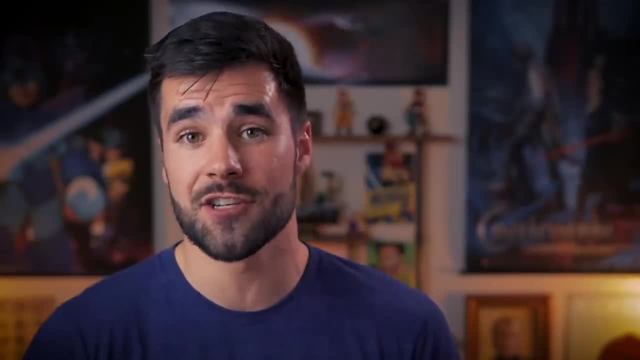 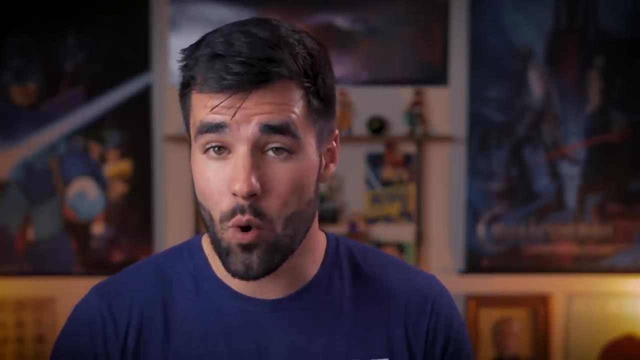 on the stove. you don't want to have greasy or meaty hands while you're trying to find your chef's knife or you're trying to find something else that's important. You want to make sure everything is in its place and you know where it's supposed to be, and it's. 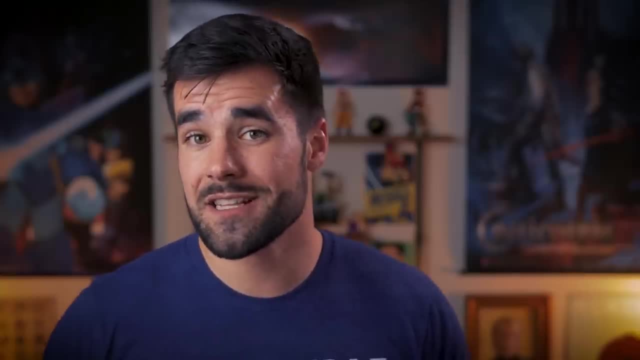 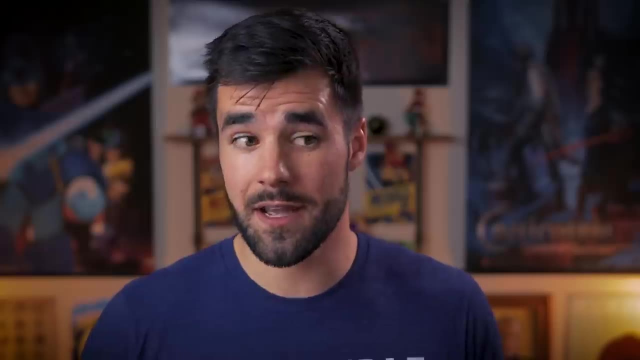 organized before you start working, And this is a concept that's not just useful in the culinary world, It's useful for anybody. Make sure that your work environment is set up properly before you begin your work And, once you're done, put things back exactly as you. 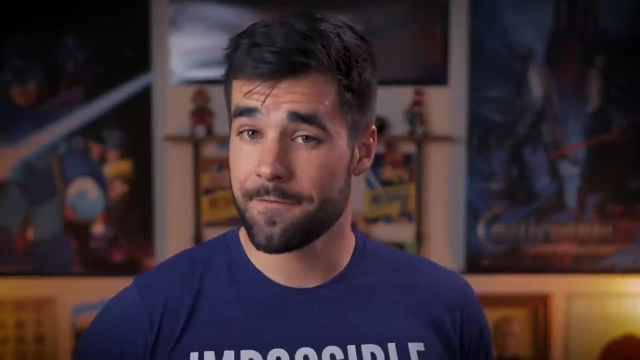 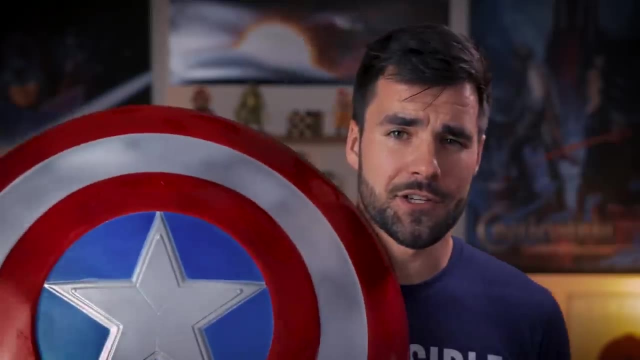 found them, as my dad constantly yelled at me to do. And finally, the list has led us inexorably to item number seven, which is worthy not of a notebook but of a Captain America shield. Organized people are very deliberate about. 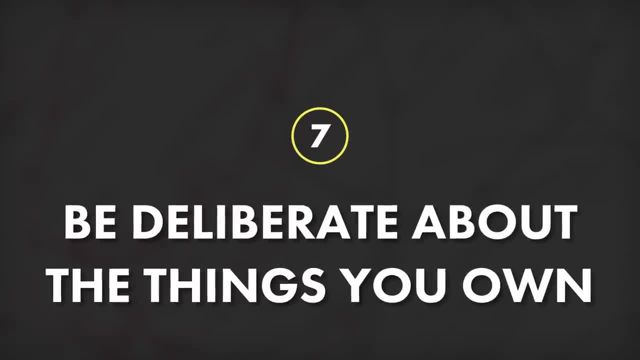 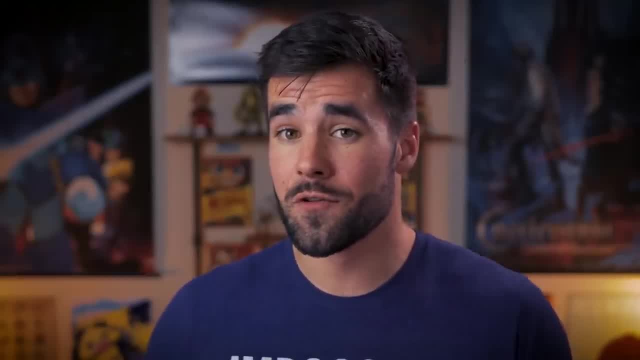 what they own, what they buy and what they choose to keep. And, of course, choosing to keep this shield was a very worthwhile decision. Now, I am not going to say that I am a minimalist mainly because my best friend, Martin, who is a minimalist and who runs my website, would. 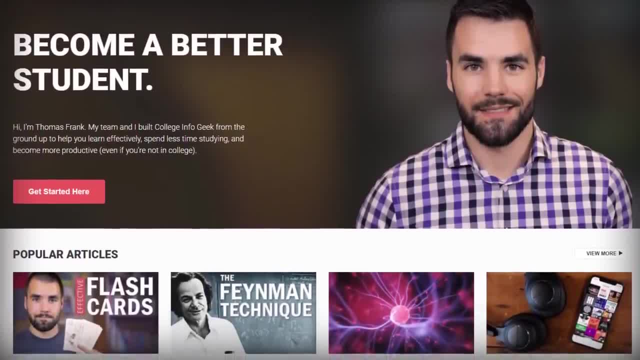 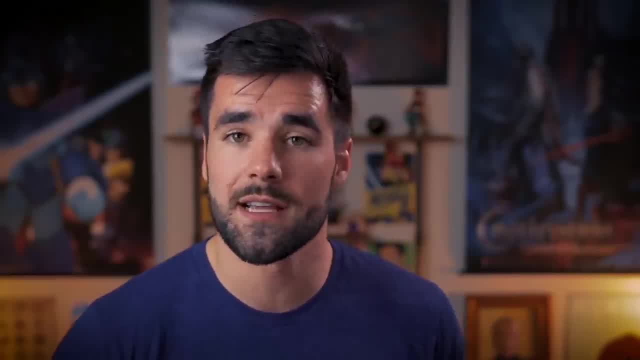 probably hack my website and destroy it- if I used that term just out of pure annoyance- But I do take care to buy things that bring me value, that bring me joy or utility. I don't keep things around if they're not useful to me. I don't let them clutter up my space, And I think this is something. 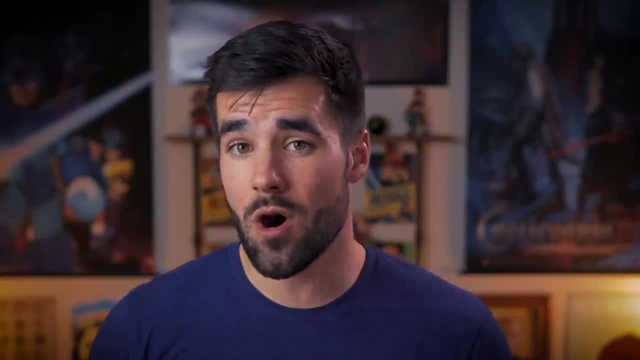 that you should keep in mind as well, Because, remember, the more things that you own, the more energy and time you have to spend maintaining them and storing them and keeping them organized, And it's a good thing to remember that organized people don't spend more time and energy than 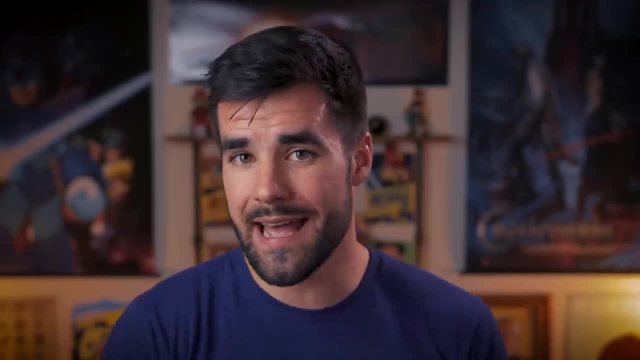 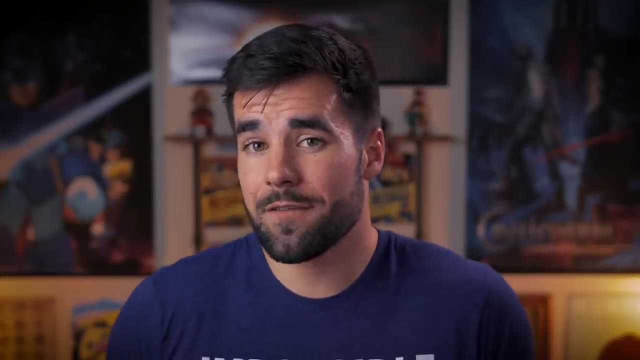 they have to. on organization, It's a means to an end. So be deliberate about the things that you buy. Ask yourself: am I buying this because it will bring me joy or utility, Or am I buying it for some frivolous, stupid reason? Or am 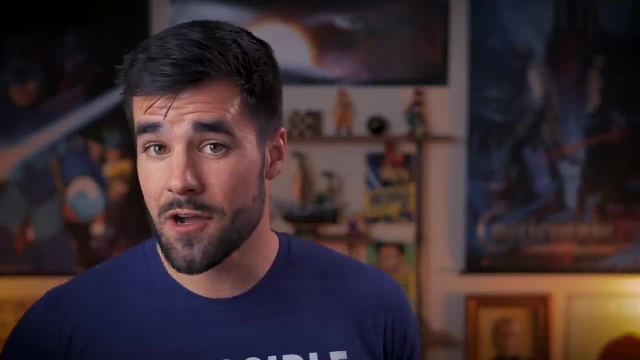 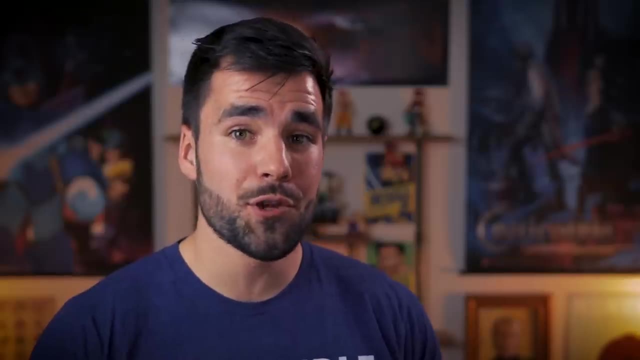 I buying it just to impress somebody else, And, likewise with the things you already own, be asking yourself on a regular basis: do I still need to keep this thing? Could I donate it to somebody else? Could somebody else get more use out of it than I could? 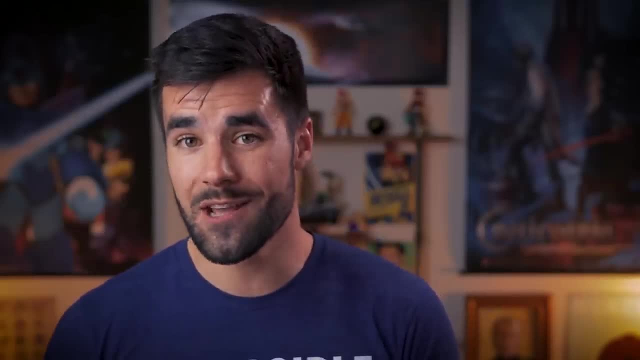 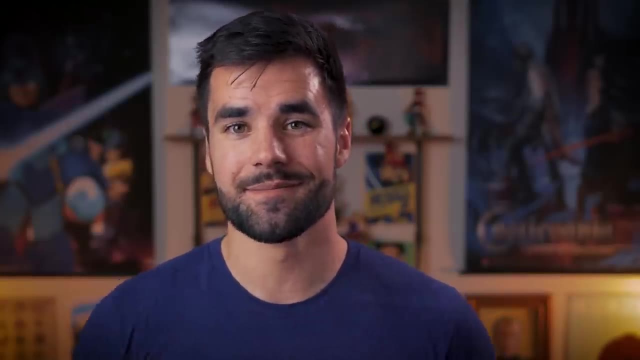 Or can I just get rid of it because it's no longer valuable to me or anyone? Do that along with the other six things I've mentioned in this video, and you will be well on your way to becoming an organized person Now, at an earlier point in this video, I talked 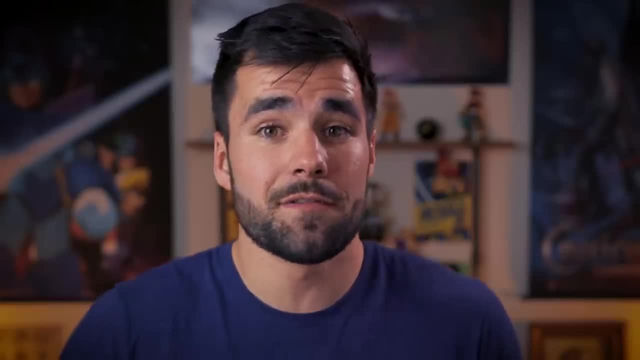 about a concept that I like to call an organized person. Now, at an earlier point in this video, I talked about a concept that I like to call the mindfulness loop. This is the process of constantly checking through the different areas of your life and making sure that their 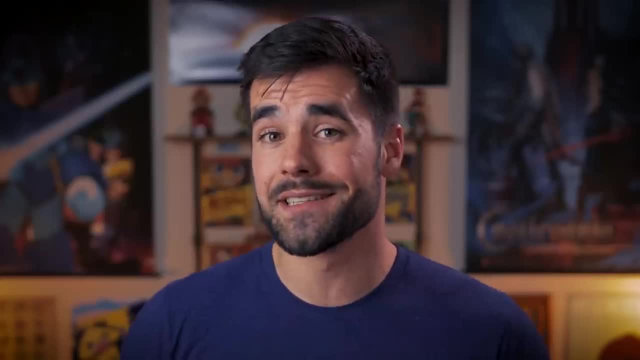 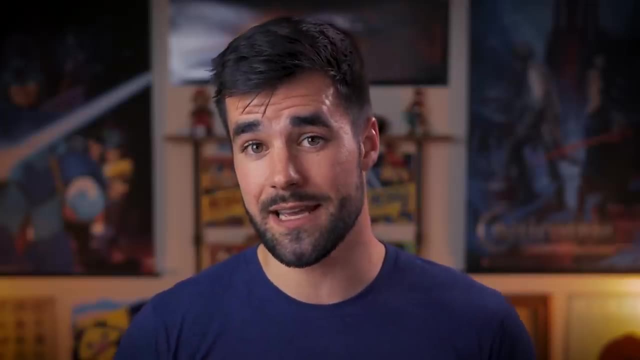 dependencies are taken care of. But the mindfulness loop actually has different levels. At its lowest level, this tool is simply concerned with maintenance, with maintaining the state of your life as it currently is, But at a more advanced level, it's also looking forward. 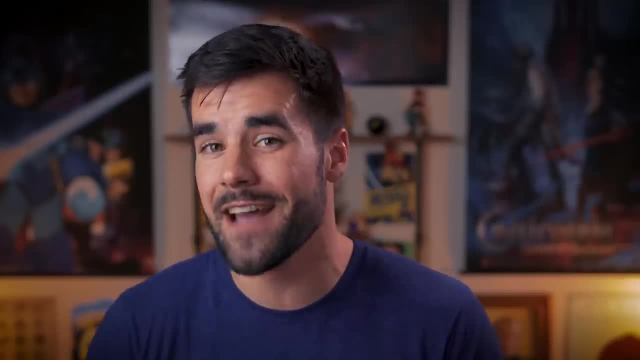 constantly prompting you with questions about what you could do to set yourself up to take advantage of future opportunities And if you want to put yourself in a place to take advantage of a wide array of those opportunities you're going to want to set yourself up to. 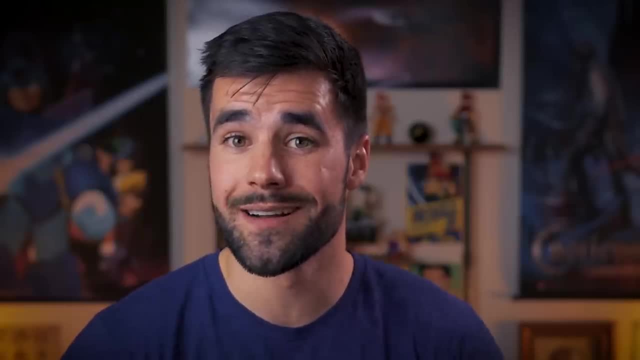 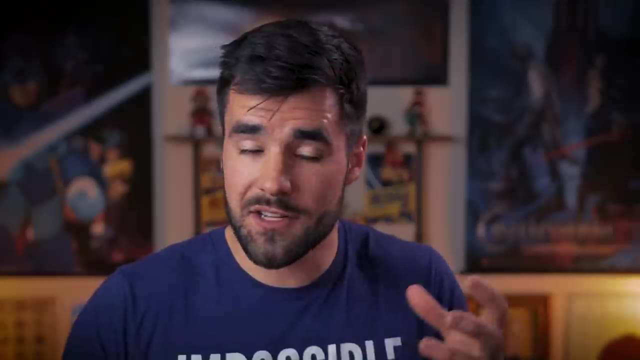 take advantage of future opportunities. And if you want to put yourself in a place to take advantage of future opportunities, then one of the cognitive skills you're probably going to want to work on is that of lateral thinking. Lateral thinking is the process of solving problems using indirect lines of reasoning. It requires lots of creativity. 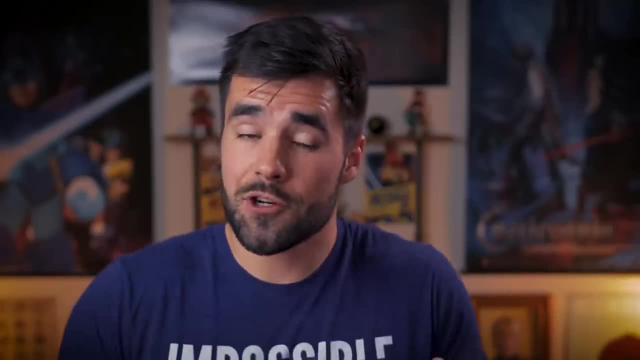 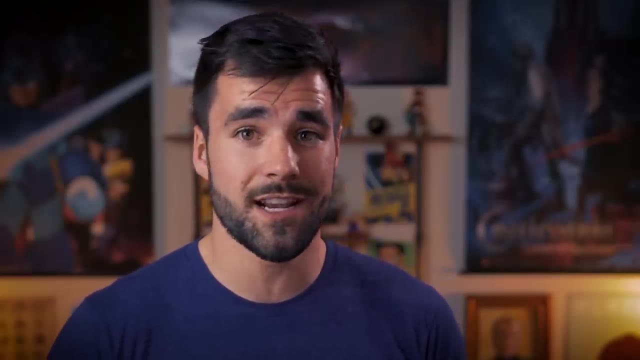 and also requires a wide interconnected base of knowledge. Unfortunately, both of these things can be acquired through practice, And if you're looking for a resource that can efficiently give you practice in both of these areas at once, check out Brilliant. Brilliant is an excellent learning resource for anyone who wants to boost their skills in math science. 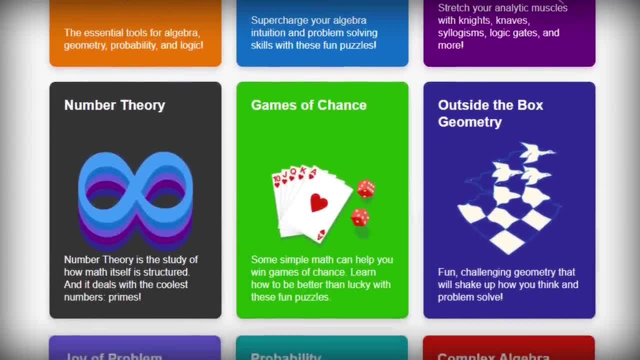 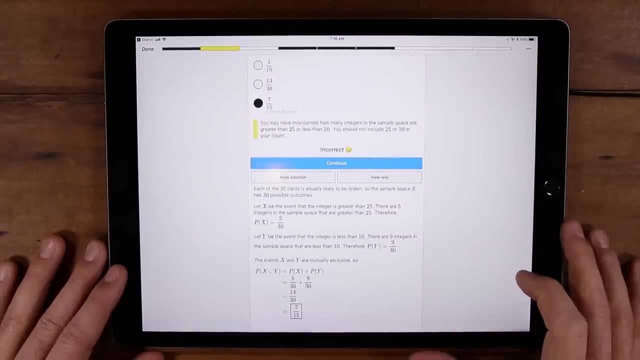 and computer science, And because they tackle all of their course design using the principle of active learning, you're gonna find yourself immediately thrown into the challenging problems that help you to build that skill of lateral thinking while you're boosting your skills in calculus, in gravitational physics, in computer algorithms. 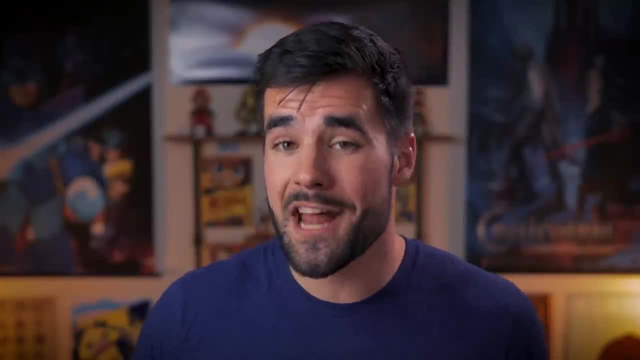 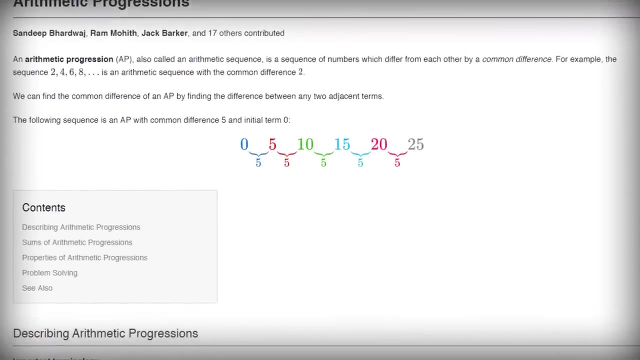 and many other topics, And even though the problems are tough, they're split into manageable chunks that aren't going to frustrate you And when you do, inevitably get stuck. there's also an incredibly detailed wiki with lots of example problems where you can go boost your knowledge. 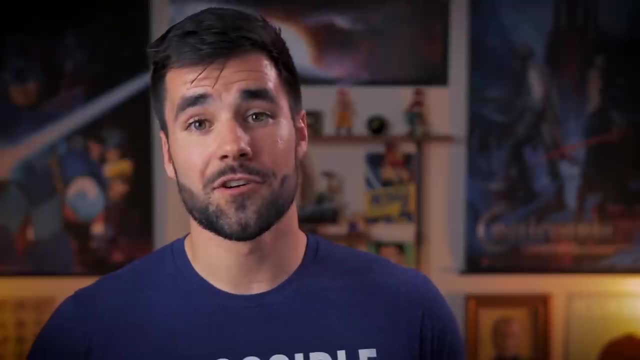 and bring it back to the problems to make sure that you can actually solve them. If you wanna start learning for free on Brilliant today, you can go over to brilliantorg, slash thomasfrank And if you're one of the first 83 people,